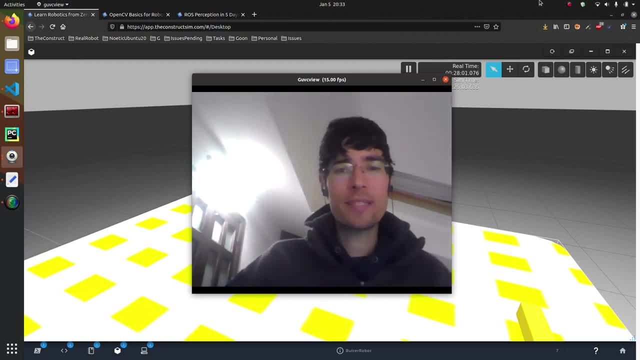 Hi and welcome to this new video on robotic basic theory. So in this video we're going to talk about robotics perception. So why do we need it? So perception is what allows the robot to not stumble upon people, to detect objects in a way that they can grab them, that they can avoid them. also, detect people so they can follow them, they can talk to them, they can. 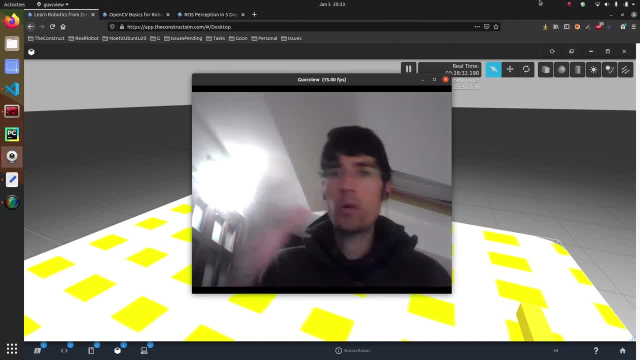 recognize who is his boss and who is someone that he doesn't know. All those things is what perception does, and much, much more, and it's very linked with AI. especially nowadays, It's basically AI all over the place. So in this video, we're going to introduce a very basic concept, which is hard cascades that are used for 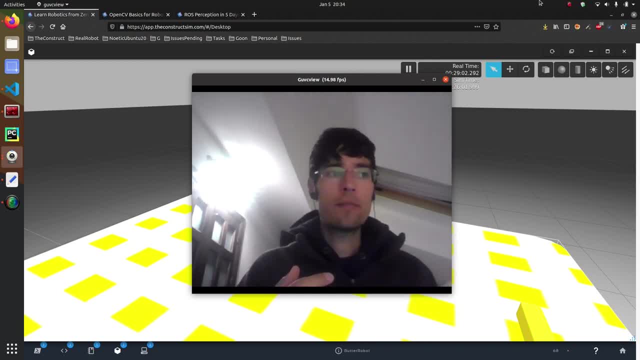 detect and recognize different kind of objects or things like human faces, which is the example that we're going to do, but it's used to detect apples, or a table or a car or anything, absolutely anything. So how does it work? Essentially, what it does is we stack- very simple. 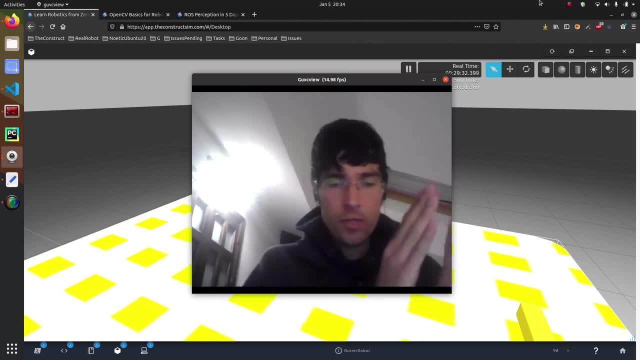 feature detections and we stack them one after the other and this group of detections make a very much more complex detection. So, for example, the face that we're going to do right now- So it's a combination of different features- which is a very basic feature- is the mouth, which is a horizontal black line cut, and then there's white on top. 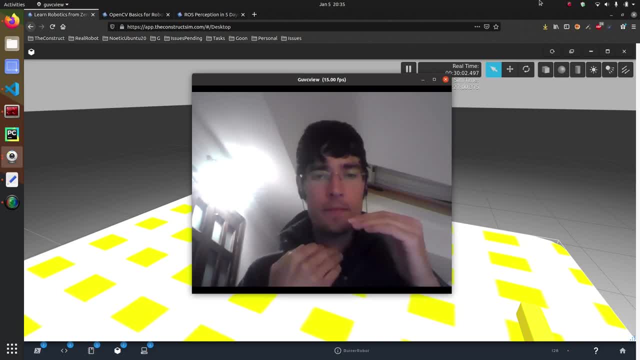 and dark and then white again. Then the eyes is basically dark, then white, then dark horizontally, and then the nose is, for example, dark, dark and white in the middle. And based on those very simple features, if we stack them together and we make detections, we can then see, okay, the object that I'm seeing. is it a face? Okay, does it have this line? Yeah, 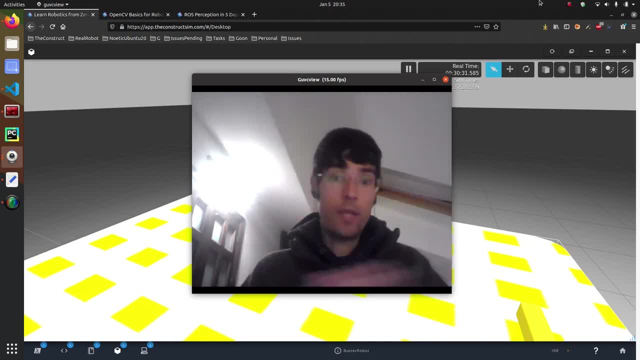 Does it have this one? I'm not sure. Does it have this one? No, Then it's not a face, For example. it's a very, very over the top explanation, but I leave in the video description links much more detailed than this that go into all the details on how this works. But essentially it's that. So what's the advantage? The advantage is that it's very 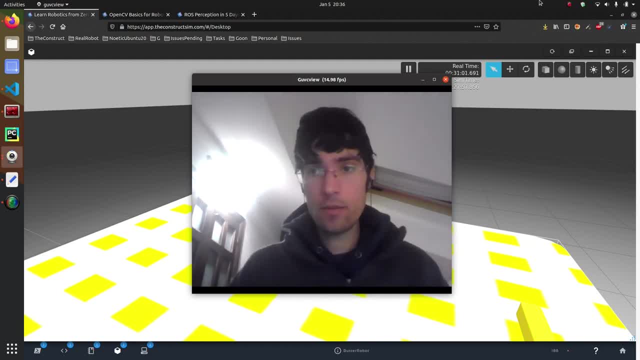 fast. It's really really fast because there's no real learning there, There's no big computers needed for that, and you can do it real time. The drawback of that is that you need to define a hard cascade file for each of the objects that you want to detect. So if I want to detect a face- human face- okay, I can detect any human face- Great. But it doesn't allow me to detect. 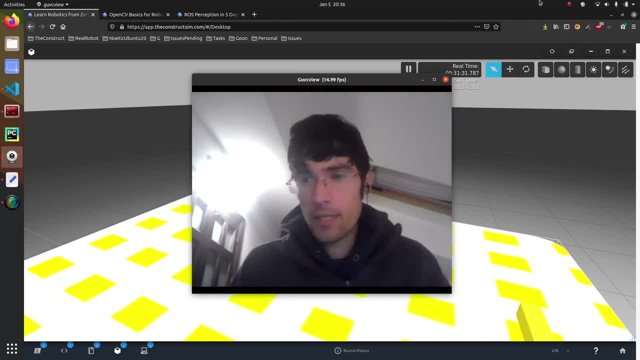 dog faces, for example, or it doesn't allow me to maybe detect cartoon faces. And obviously, if I want to detect another thing like an apple, I can't recital it. I have to generate a new one which is generated by AI, deep learning systems and all that stuff. So, depending on your application, it's really good. If you want a more generic solution, it's not the solution. 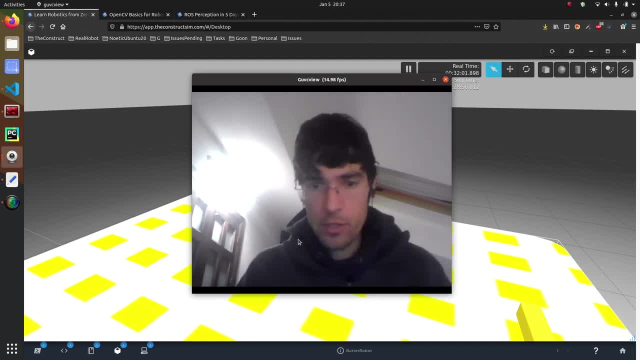 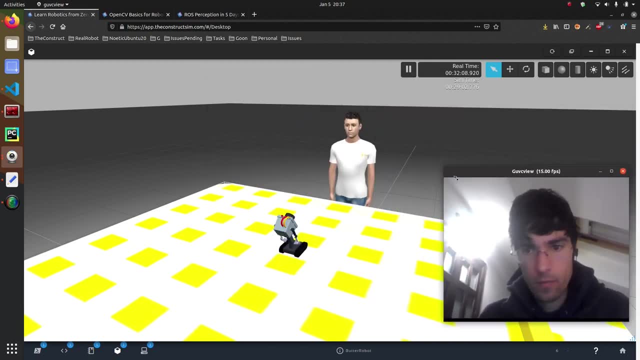 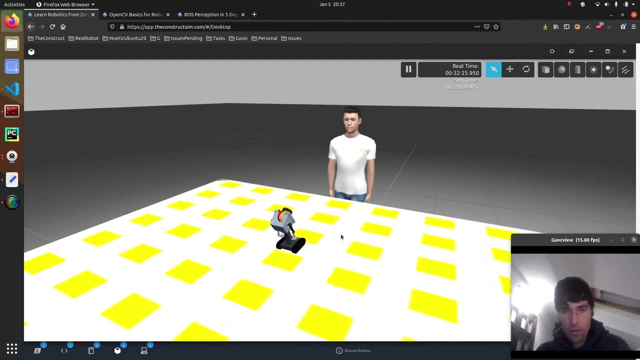 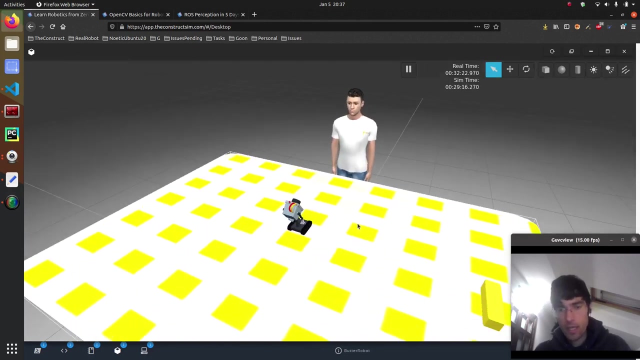 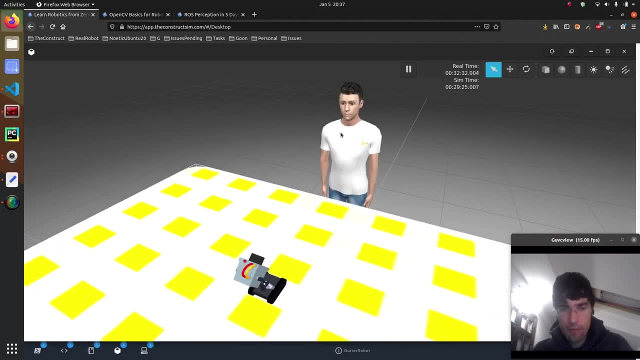 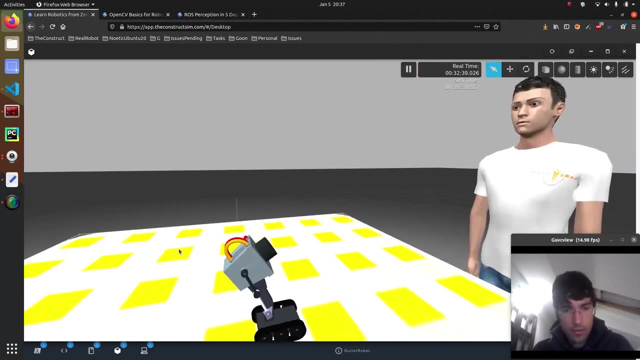 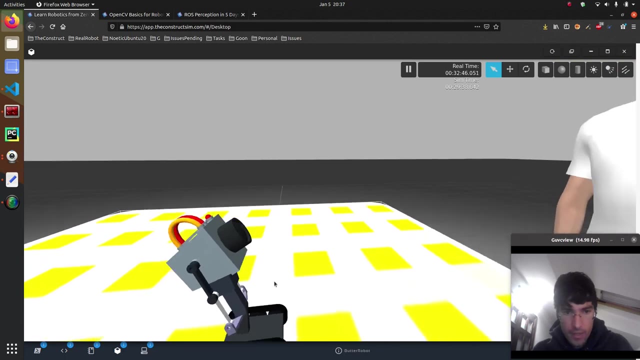 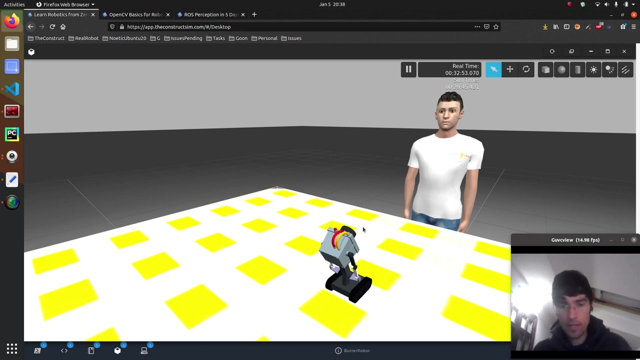 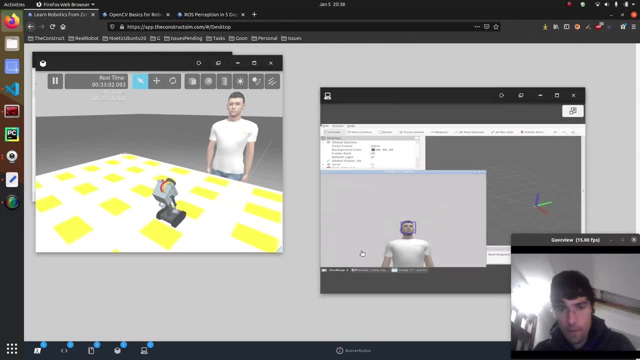 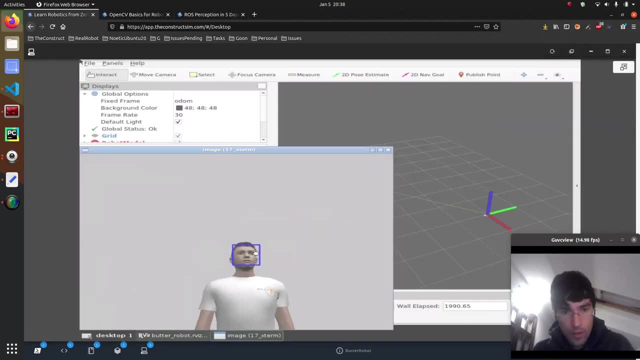 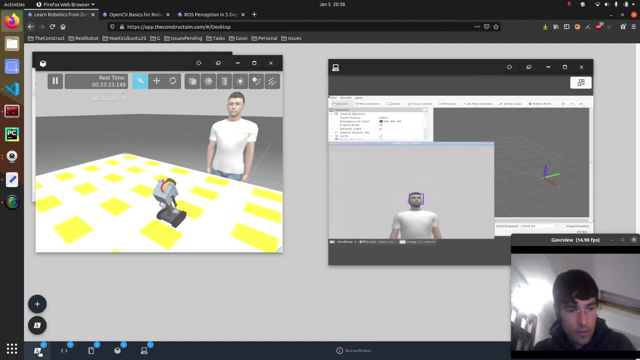 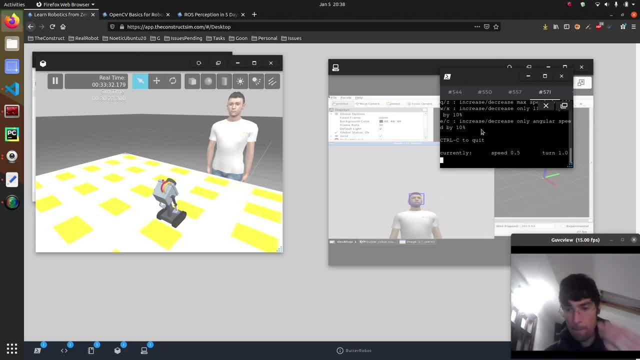 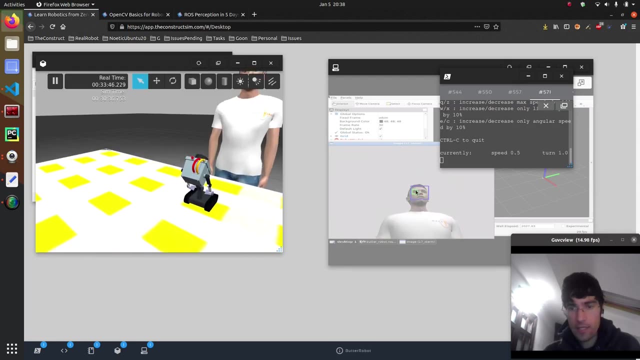 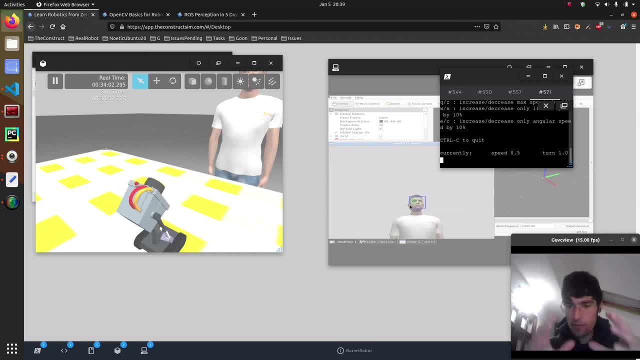 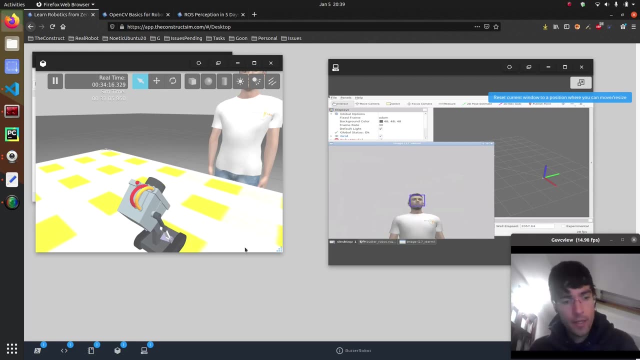 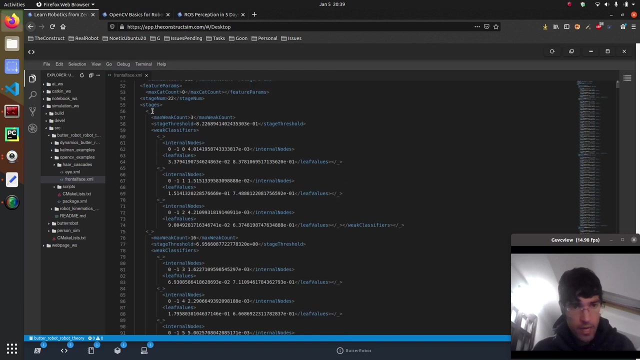 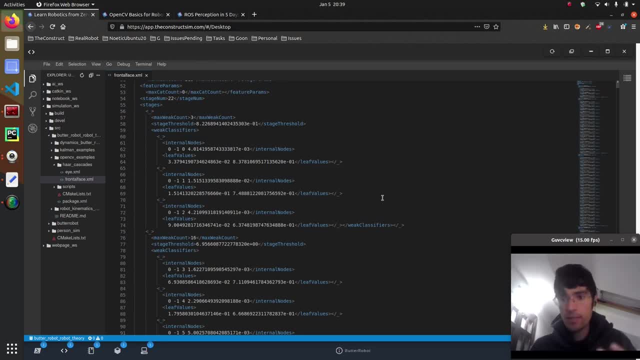 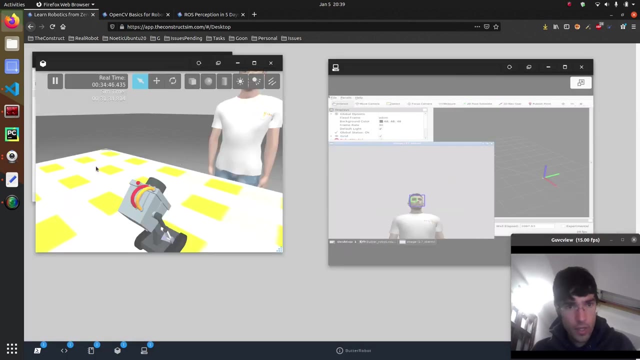 real representation of what the robot would be, And in this case, I've scaled it so that it's a more real representation of what the robot would be. And in this case, I've scaled it so that it's a more real representation of what the robot would be And in this case, I've scaled it so that it's a more real 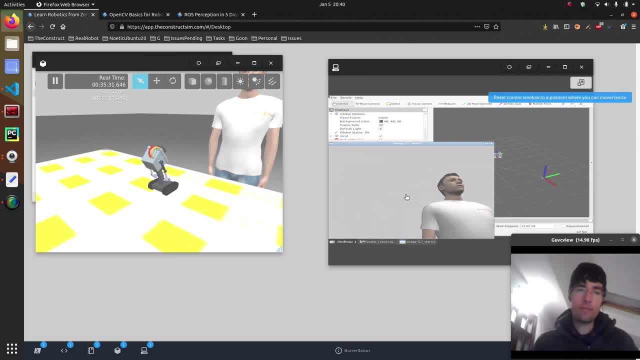 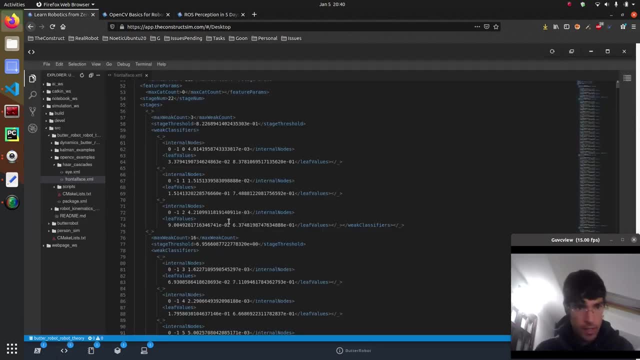 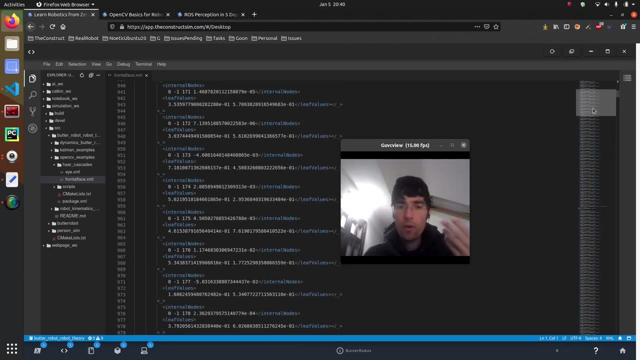 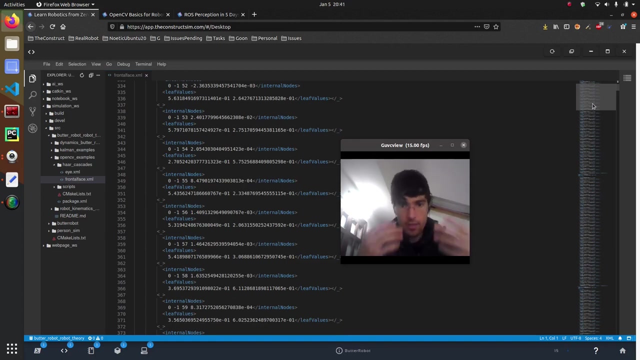 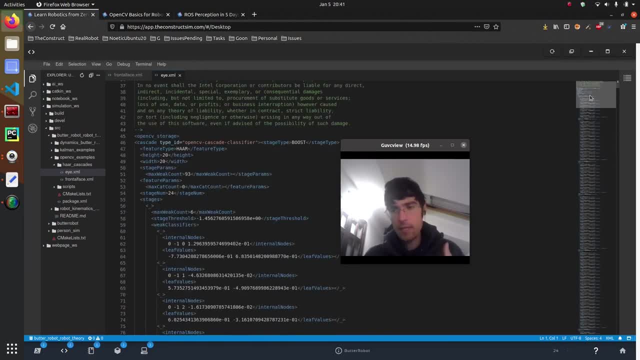 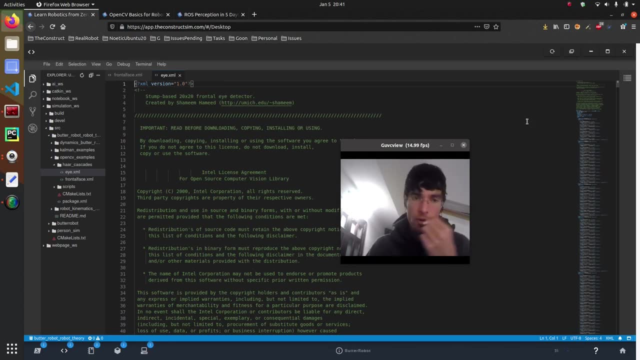 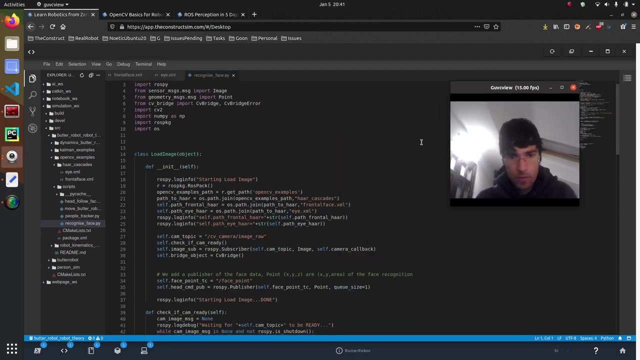 again, super long, super complex, but normally you can find higher cascades for a lot of things already done for you, so normally you don't have to create them. so, and just to give a more detail on how this works, essentially what we have is this recognize phase file running, which what we have is: 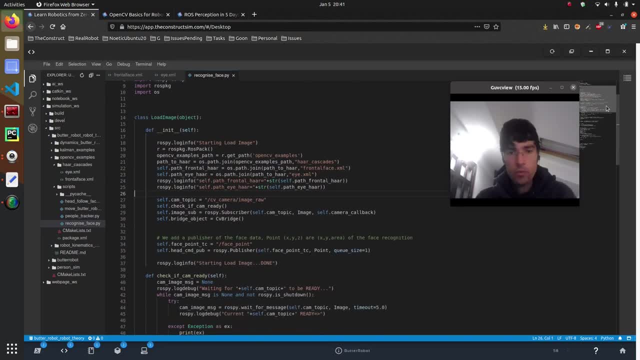 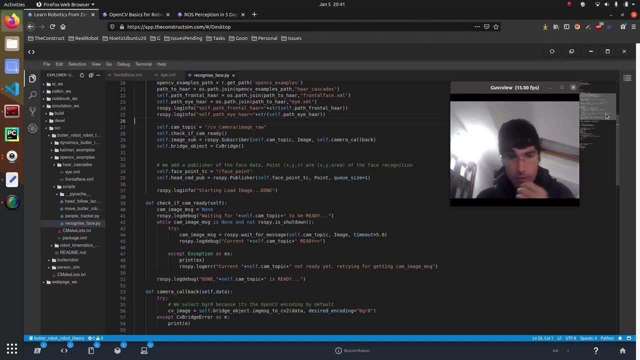 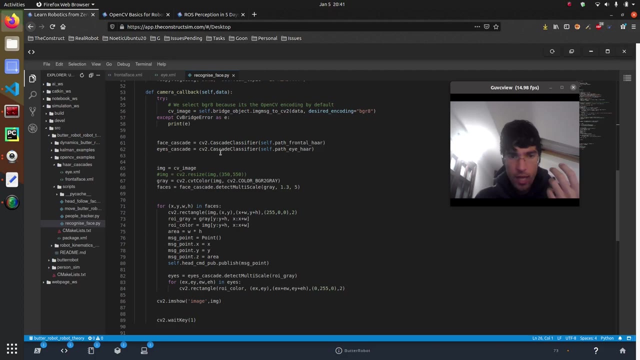 it's using OpenCV to get the images from Ross simulation or Ross system. it could be a real robot, doesn't matter. and what it does is get the image and it gets. it passes that image through the cascades, the cascade classifier, and boom, it has it. so, basically, it gets the image. 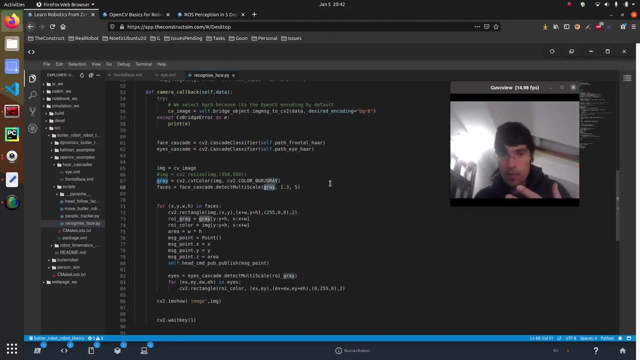 it turns it into grayscale, because hard cascade, in this case, doesn't use colors, so it would be a waste of resources. so it's a grayscale, and then it just detects faces, and the same happens with the eyes. the same thing. so here you. you have the eyes detected. 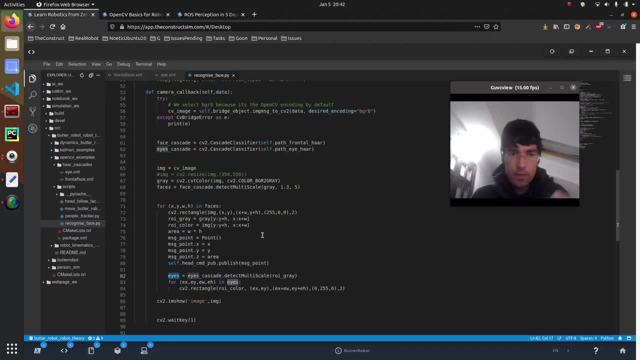 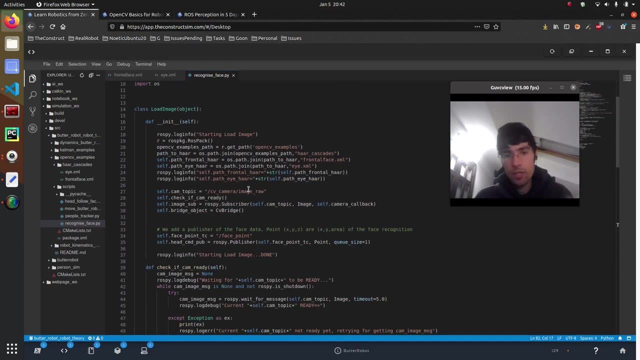 that's it. so it seems pretty simple. so for using it, it's really simple. for developing, it's not that simple to do it, and then this one is detecting the faces and then it's publishing a topic that does that. yeah, so if you want to learn more about an 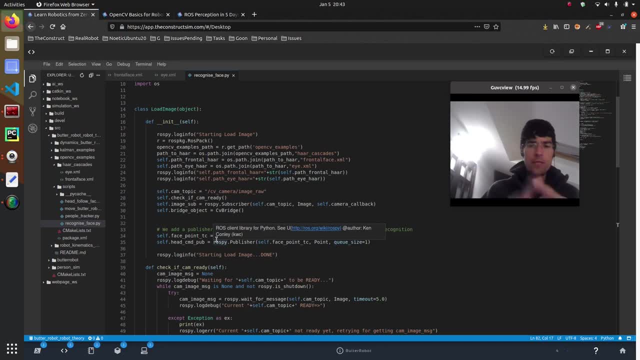 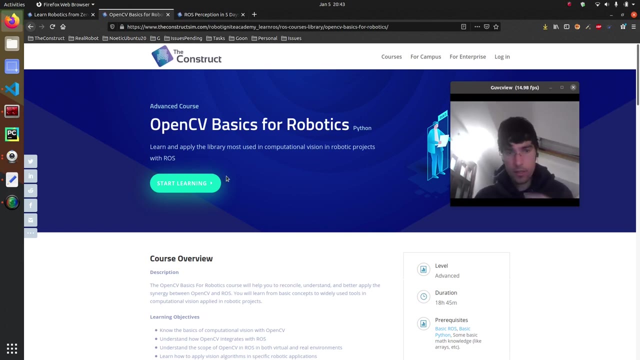 open CV- not only face detection but people tracking or object detection or AR tags and so on. I highly recommend you that you do this course on open CV basics in the construct and I followed these this course previously to do this video and it really helped me a lot to have this.